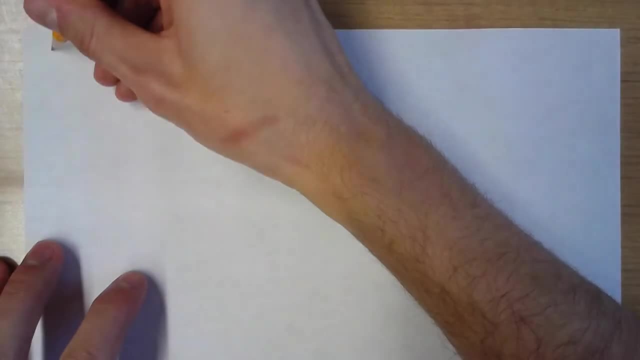 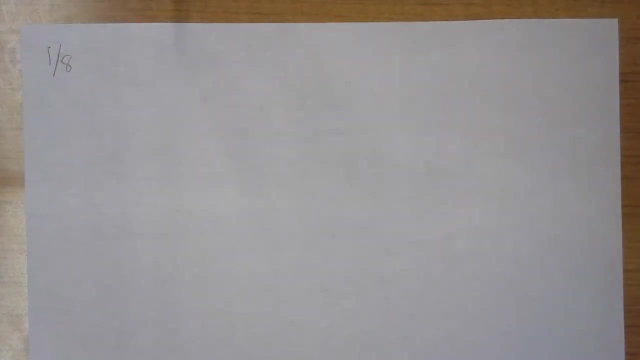 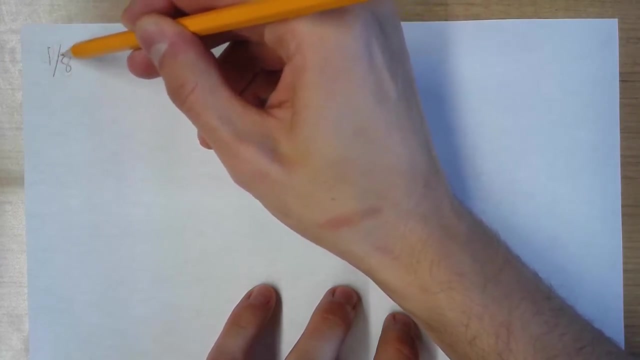 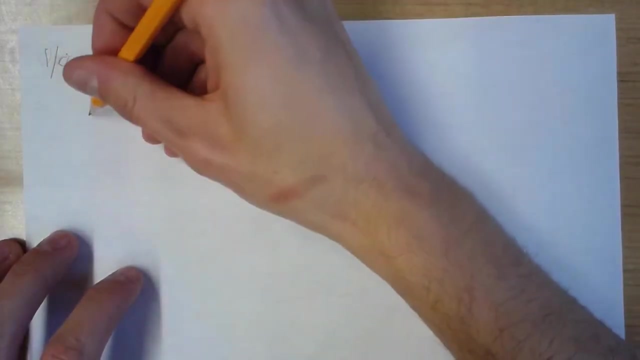 So let's look at a couple of different examples. The first example I want to go through is 1 eighth. Now, as we know, a fraction is also, similarly, a division symbol. if we divide this number here by this number here We divide the numerator by the denominator. So how do we divide this? Very simple, We know that the bottom number is what is on the outside. always, The denominator is always on the outside. 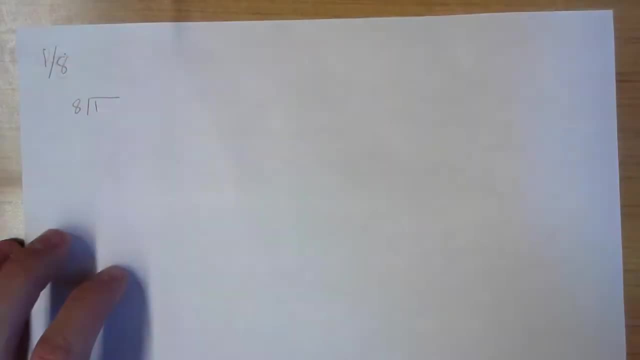 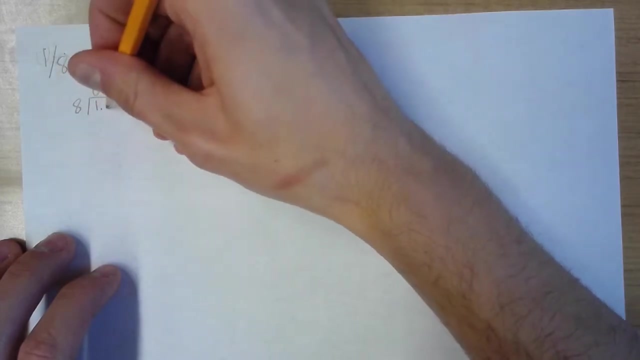 And it's dividing into our 1 right here. So long division. we know the process Very straightforward. So we know that 8 goes into 1 zero times. So we have to add a zero here, because you're going to always add as many imaginary zeros as you want at the end of a decimal place. 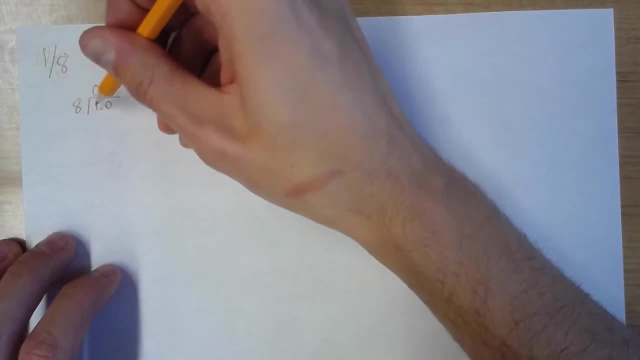 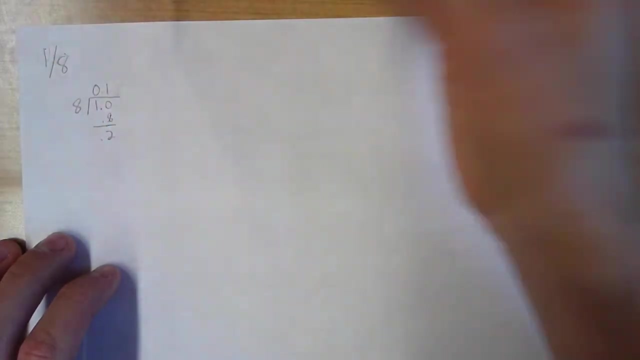 So we have: 8 goes into 1 zero times. 8 goes into 10,, 1.0 or 10, one time. So we know that we repeat the process. We have 1, 8 goes in once, which is 0.8.. So what we are left with on this side is 0.2.. Now we repeat the process one more time. 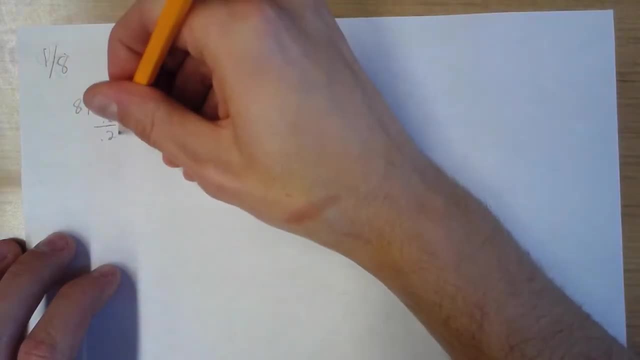 How many times does 8 go into 0.2? It goes in zero times. But how many times is 8?? If we add in another imaginary zero here, how many times does 8 go into 20? 8 goes into 20 two times. So what we are left with here is 0.16.. And when we subtract those together we have 0.04.. 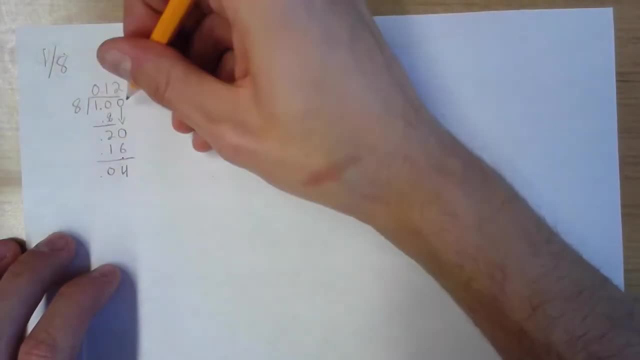 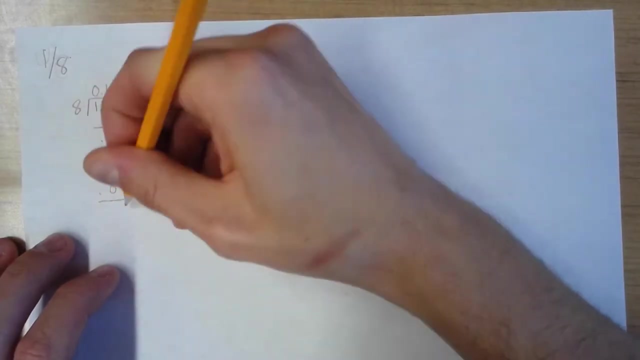 Now, 8 goes into 0.04, zero times. We know that We have to take another zero here. So we know 8 goes into 0.040, goes into 40, five times. So what we are left with here is 0 or 0. And we are left with zero. We have our answer So, which is 1, 8 equals 0.125. 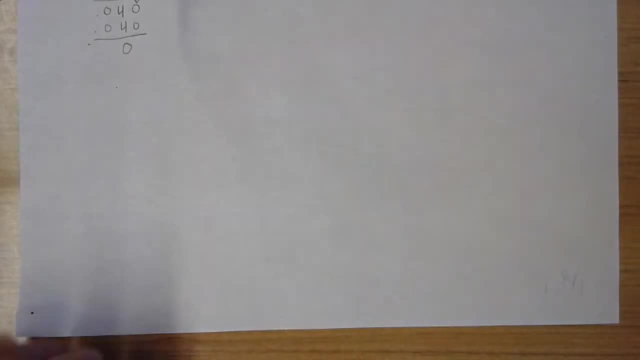 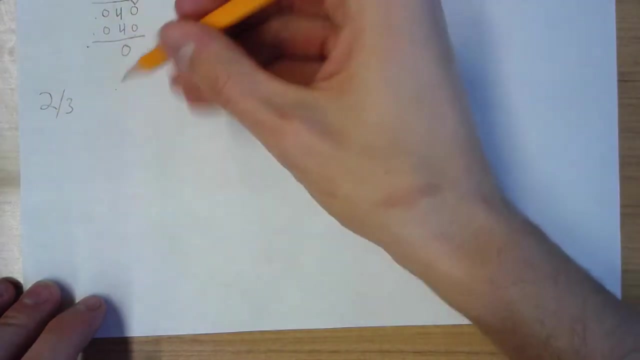 Now, our first example was really straightforward. But what if we had a different looking fraction that we were trying to make into a decimal? Let's try two-thirds. So we are dividing 2 by 3.. The numerator is being divided by the denominator, So we are going to follow the same steps here. 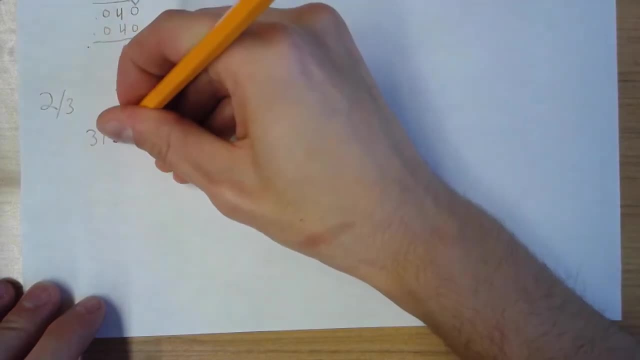 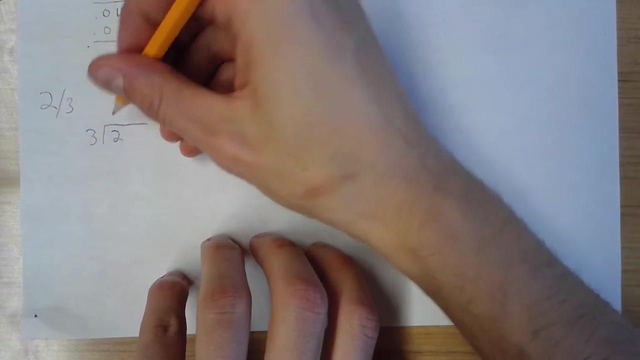 We have 3 on the outside and then a 2 on the inside, So we go through the exact same steps. How many times does 3 go into 2? It goes in zero times. We bring down an imaginary zero here. 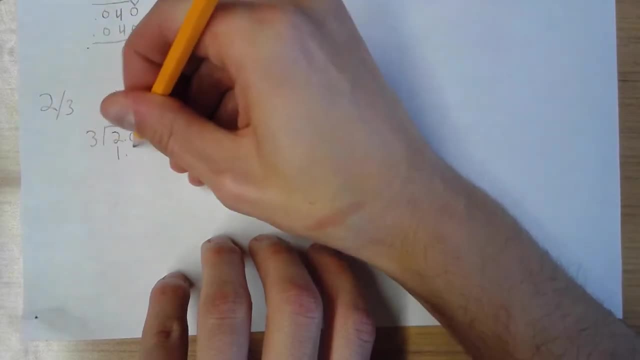 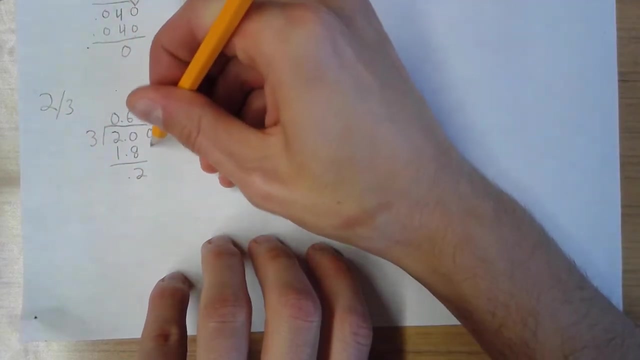 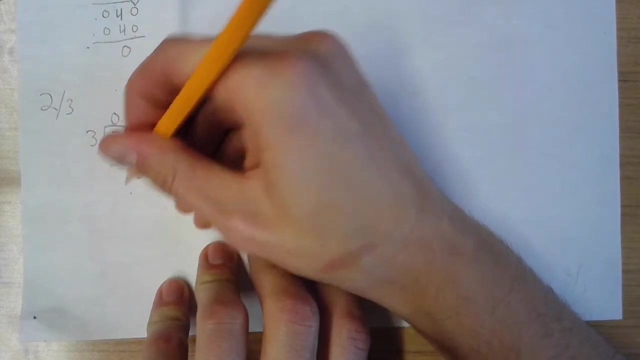 How many times does 3 go into 20?? It goes in 6 times, So we have 1.8 here. Do a little bit of subtraction. We have 0.2 here now. So follow the exact same process: 0.2, add in imaginary zero. So now we have 0.18, because it goes in 6 times, So we have another 0.02.. 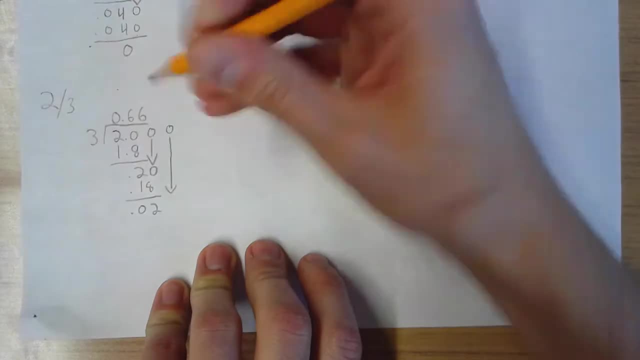 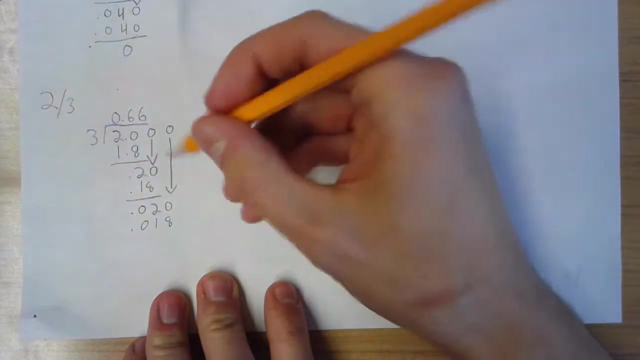 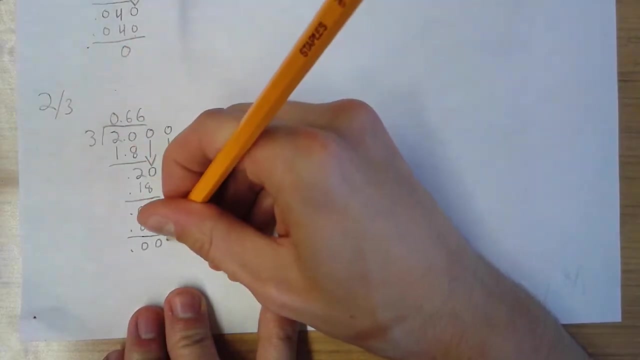 Now, if you notice, this repeats. We are always left with a point two or a point zero, two or just two, and then we continue to multiply our three by six to get our answer. So we always have a six up here and now. 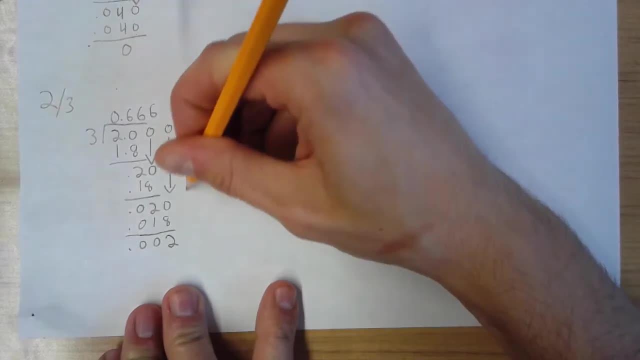 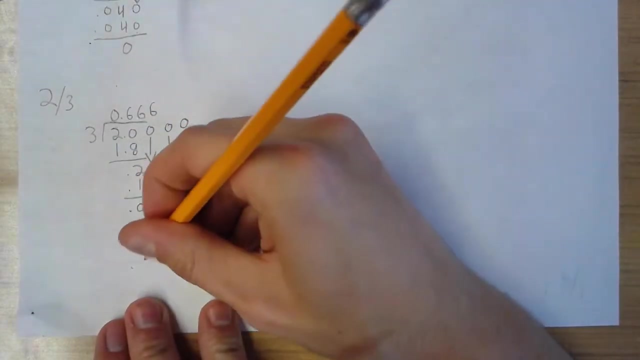 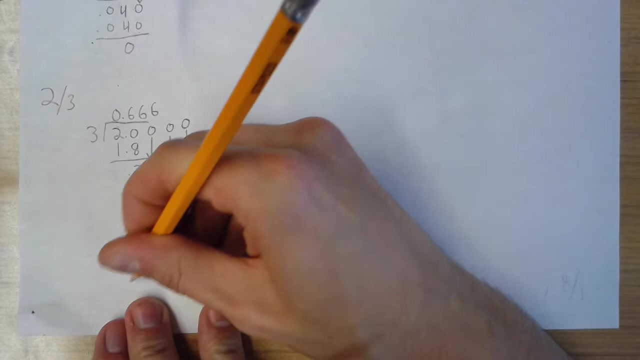 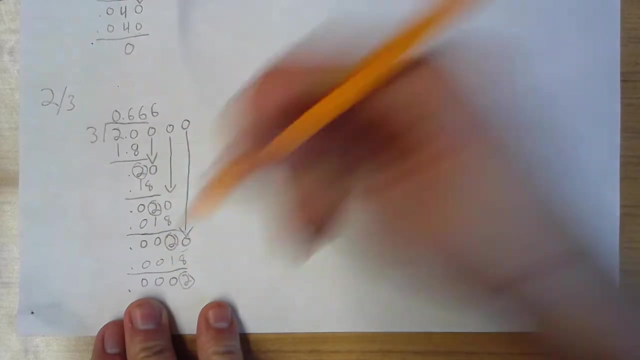 this process is never going to stop, because every time we add another zero, we are here, we're dividing three into another 20.. So what we have is, in some regard, 18.. So we have that 20 minus 18, always leaving us with a two moving further and further away into smaller places. Here it's in the tenths. 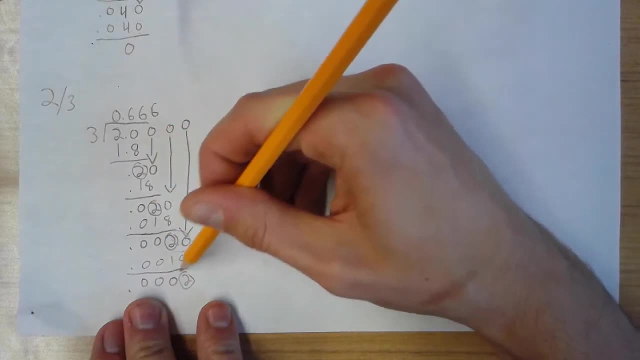 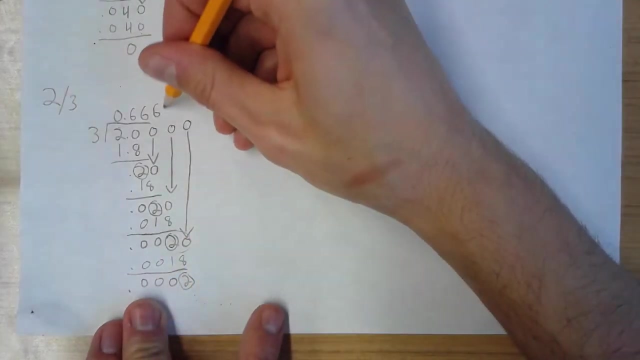 place, hundredths place, thousandths place, and then so on and so forth. So this process continues forever. So what does that mean? It means that we have a point two. So we have a point two. How do we write that? We can't just keep writing sixes forever, So there has to be an easier way. 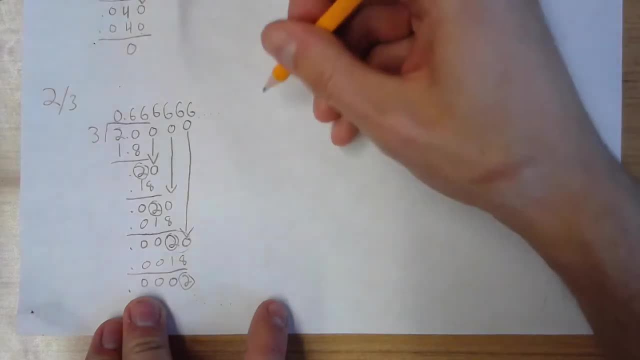 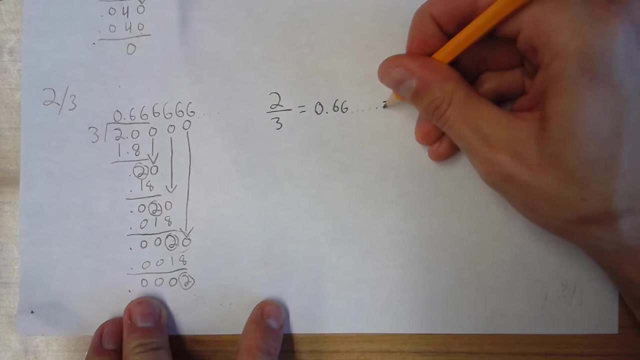 to write this. So we know the sixes will go on forever. There's another form that we can write this to simplify our answer: Two-thirds is going to equal 0.66- forever. right? I have the ellipses here, meaning that this is going to go on forever. We can also write this as 0.6, with a line above. 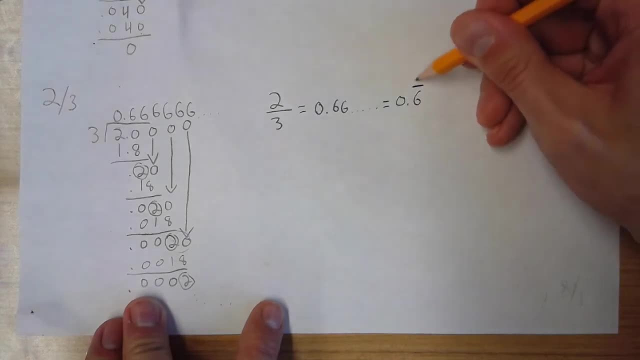 it. You might have seen this symbol before. This infers that we are repeating the digit underneath the bar here. So this is saying this is 0.6, and the sixes are going on forever. This is just an easier way to write this. Now let's go on. 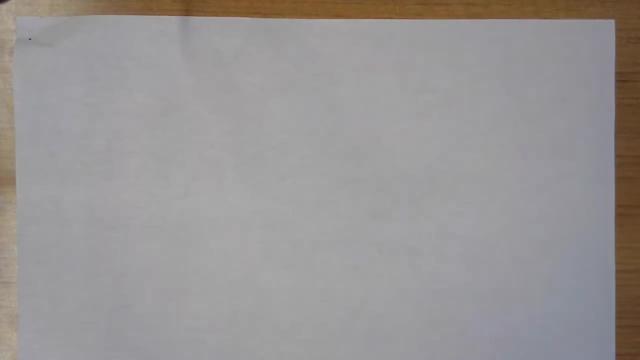 to a third example. These are going to get progressively more complicated, so I want to make sure that on this one you're really focusing, because this is a concept that is building off of the others that we have previously mentioned. So, another problem: One over 18, right So? 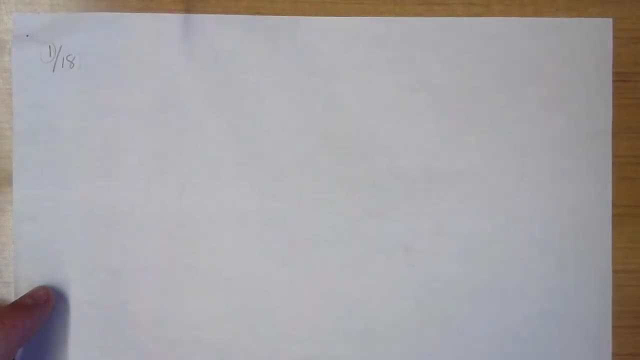 we're going to divide 18 into 1.. So we're going to go through this the exact same way we had done before: 18 is on the outside, 1 is on the inside. Now, this time, we know that 18 does not go into 1,. 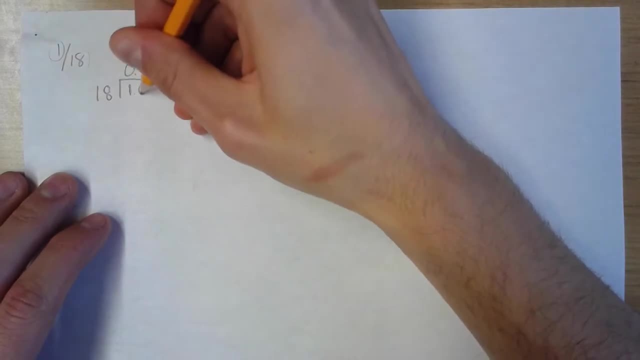 goes in 0 times, and 18 does not go into 10 after we add an imaginary 0. So we have to add another imaginary 0. So how many times does 18 go into 100? It goes in 5 times. So what we're left with here is a 0.90, and so we minus that out. So we have 0.10 here, and 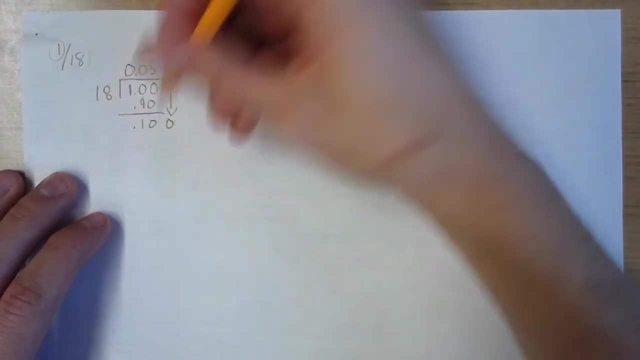 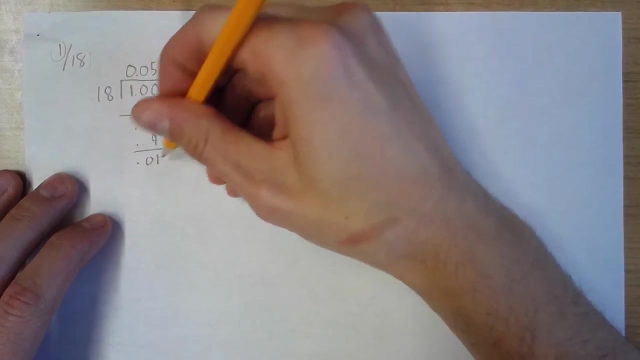 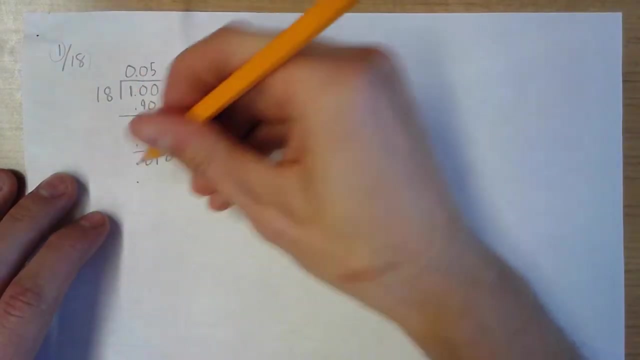 now we repeat the process again, Drop another 0 down, So we have another 100.. That is times a 0.9 and here we have 010 again And this process. I'm sure at this point you can finally recognize that it will repeat forever yet again. 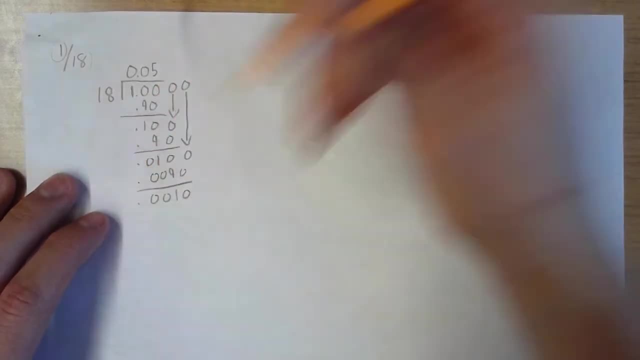 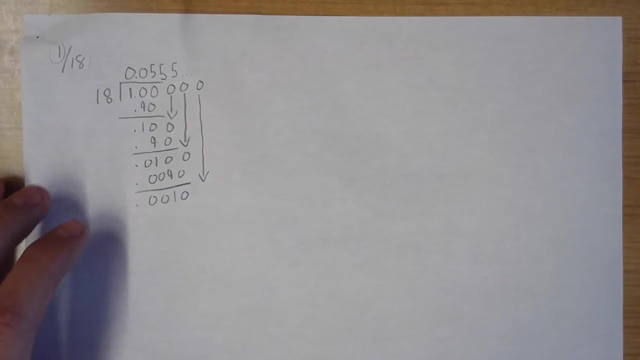 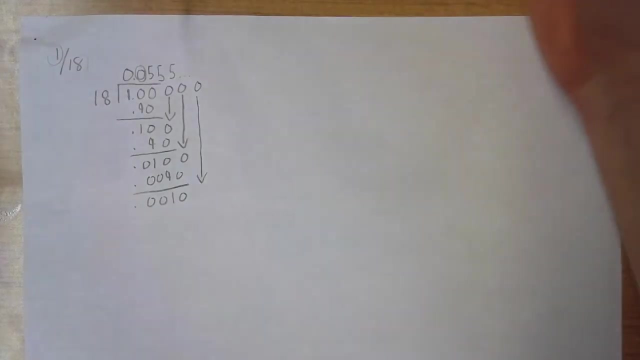 0, 0,, 1, 0. And then we just continue to do this process forever: 5, 5.. So we keep going. But you'll notice something interesting about this problem is this: 0 is not being repeated after the decimal place. 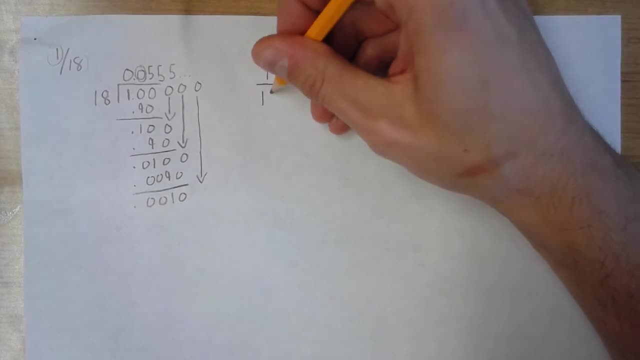 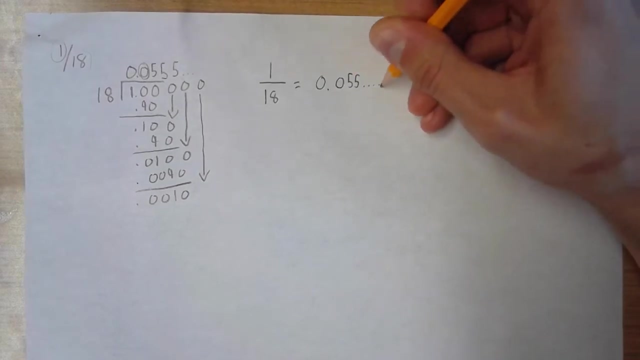 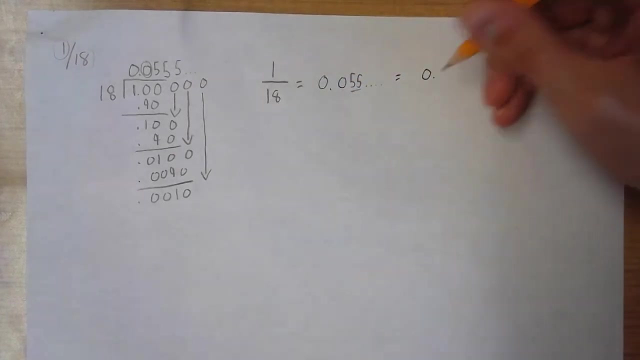 Only these 5s are. So our 1 over 18 can be simplified as 0.055 repeating, right With this 0.055 repeating and not the 0 repeating. Or it can be written as 0.05.. And our little bar that. 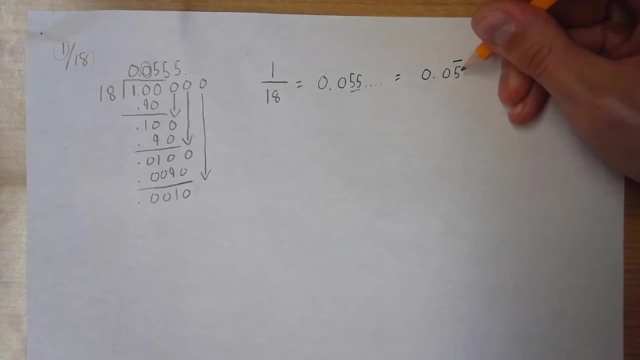 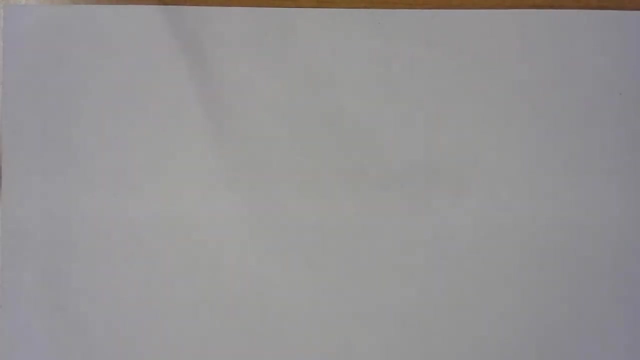 represents repeating numbers is only over the 5.. So the 0 is here first and then our 5 is what is repeating forever. All right, mom, There's just one more example I want to show you. I know these problems can kind of feel pretty long and belabored, but trust me, the process is very important Once. 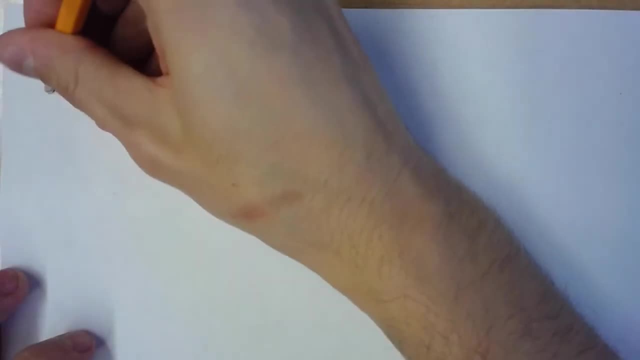 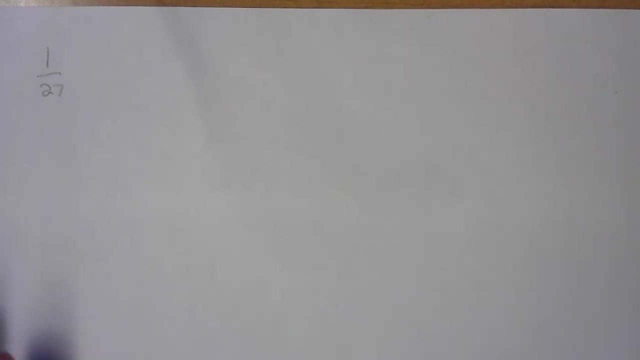 you get the whole thing together once you take the whole process down. this will help you with a lot of math in the future. Long division is a very important concept. So there was one more problem I want to do over. I want to do. 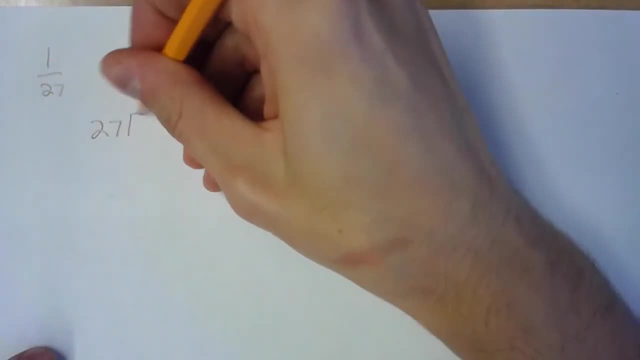 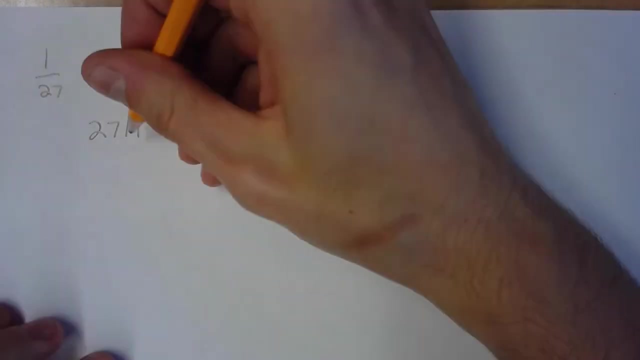 1 divided by 27.. So how is this going to look? We have 27 on the outside and then 1 on the inside. Great. So we should immediately recognize that 27 does not go into 1. And 27 also does not go into 10.. So we have to add another. 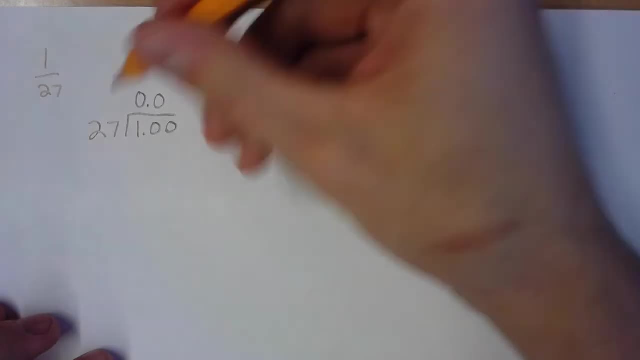 0 here And we have to add another imaginary third. So what do we do here? Let's go over that 0.075, we just divide that zero here. So how many times does 27 go into 100? It goes in three times. So 3 times 27 is going to. 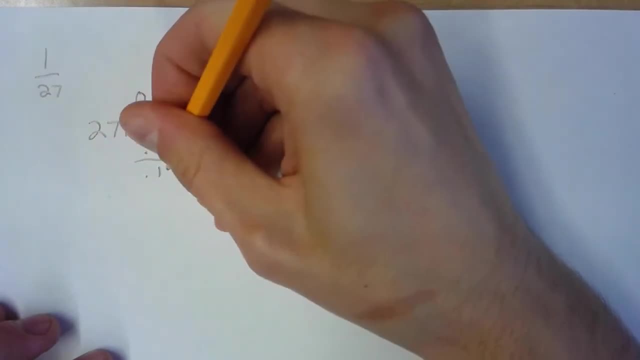 be 81.. Great, So now we just continue like a regular problem. 100 minus 81 is going to be 0.19.. We know that 19 is not divisible by 27,, so we have to add another imaginary zero here. 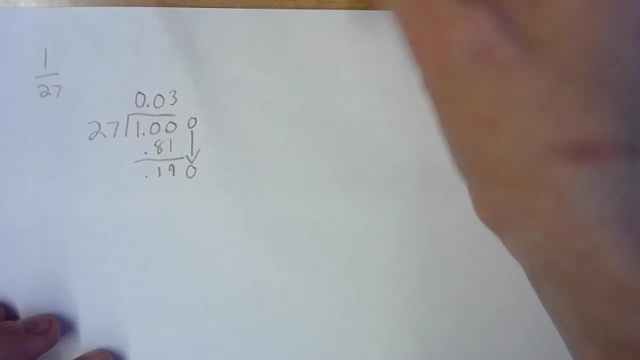 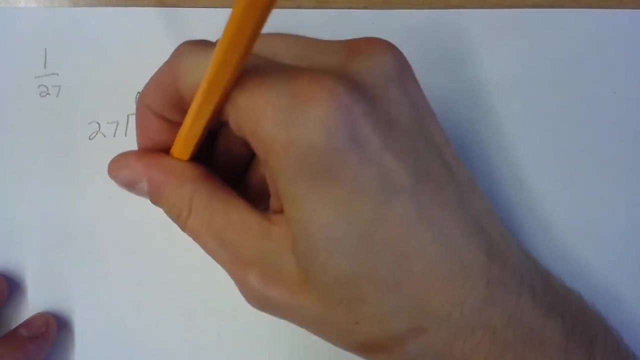 190 divided by 27.. That is going to be the closest to it would be about 7 times. 7 times 27 is going to equal 189.. So continue the process: 0.001.. 190 minus 189 equals 0.001.. Great, but we're not. 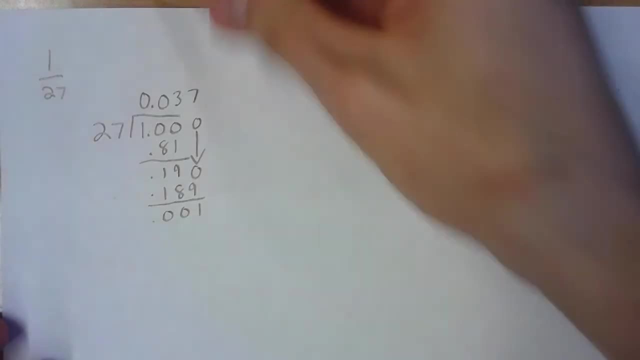 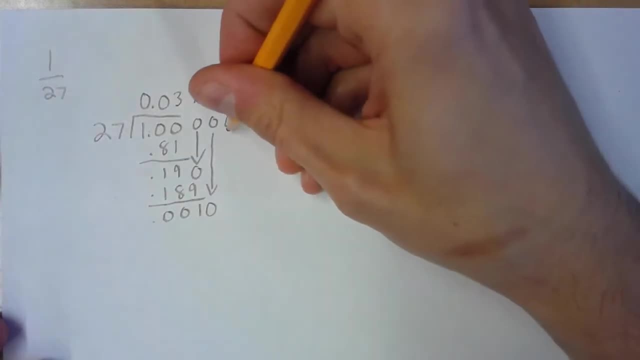 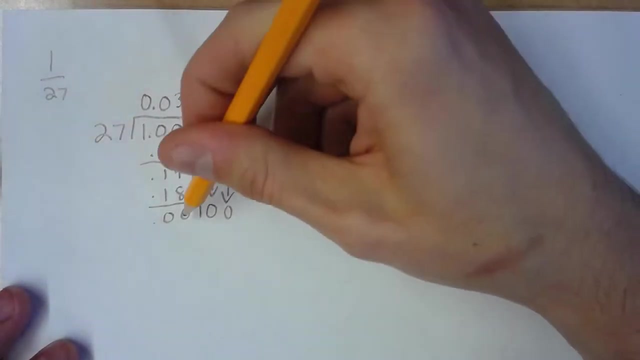 go into 1.. So we know that 27 does not go into 1.. So we know that 27 does not go into 1.. So we have to add two zeros here, And so we are adding one additional zero up here. So how many times does? 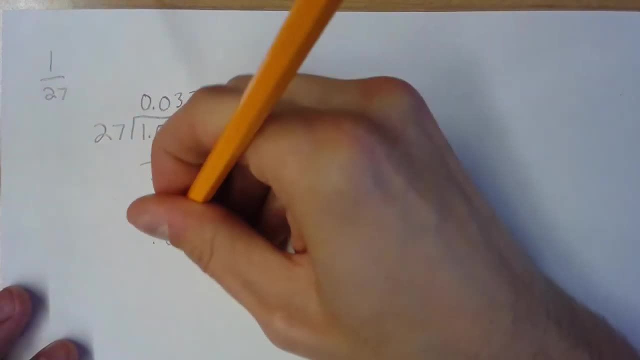 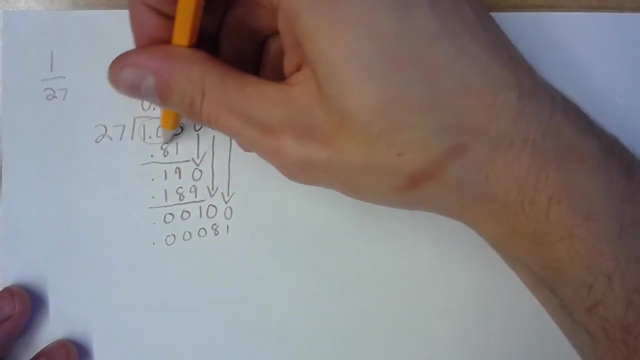 27 go into 100? It goes in again three times. Now how do I know that? This is similar to what we did at the start of our problem? We had that first 100, and then we divided that out. We. 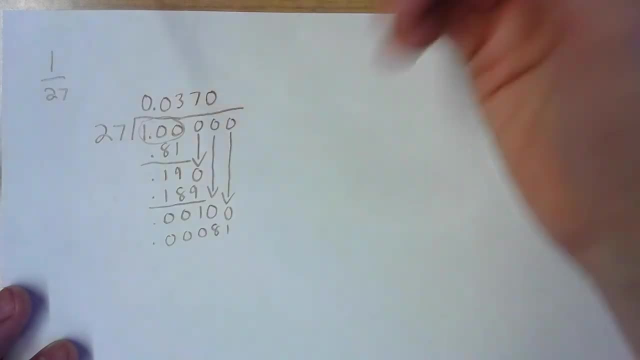 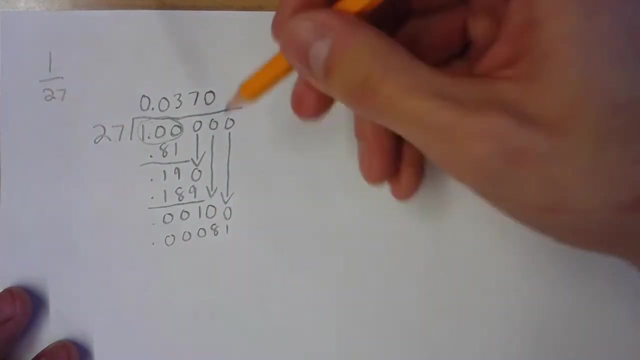 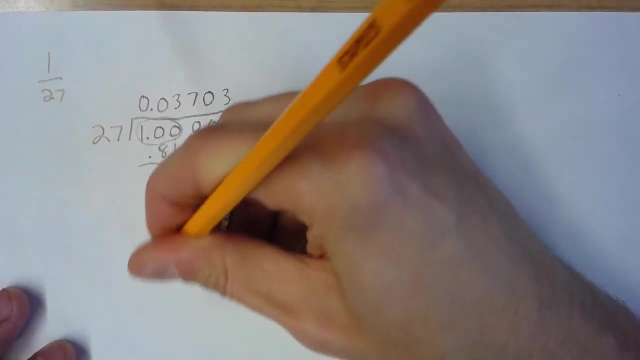 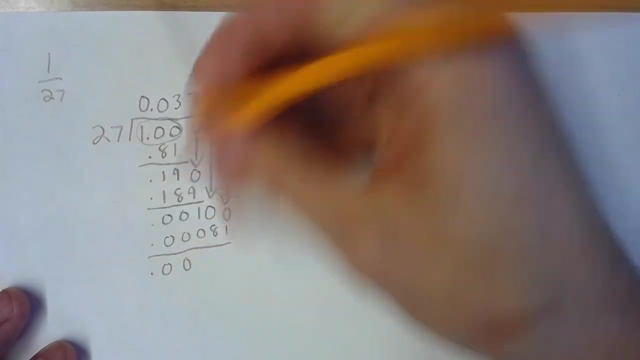 minused out 3 times 27,, which was that 81. So let's see if the process will continue. So we know that 181 is the most even number of times. 27 goes in there, which is 3 times, And now we are going to continue our process, making sure to keep in mind that we want to keep all of our numbers here in our correct columns, to make sure that we are not getting confused. 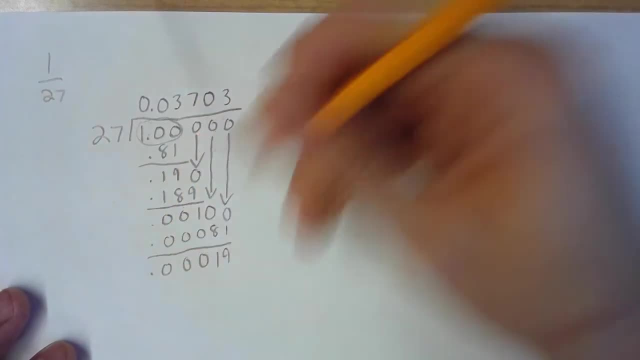 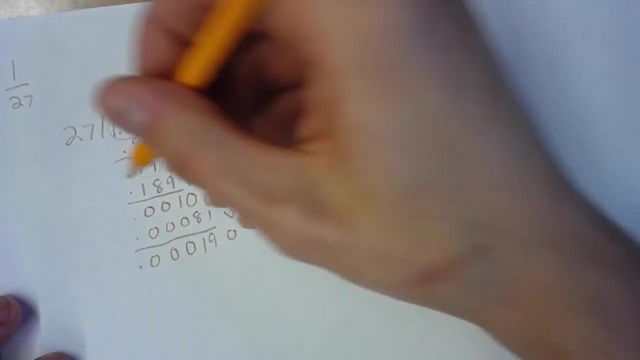 So we have 100 minus 81 is going to be 19.. Again, similar to what we have up here, 27 does not go into 19 evenly, so we have to bring down one additional zero. So now 27 goes into 190. how many times? 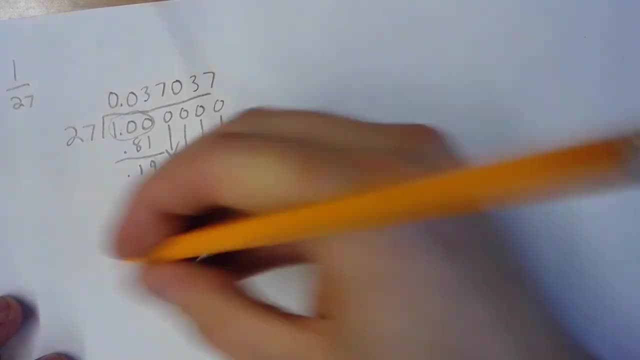 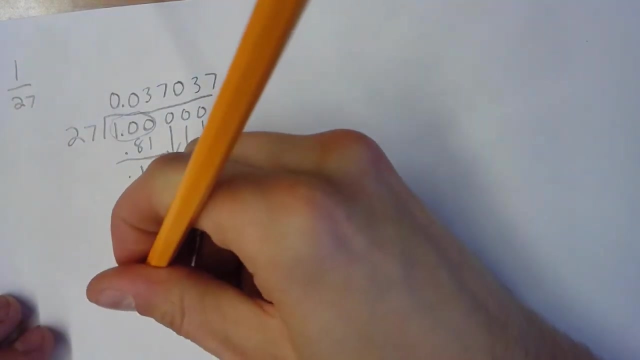 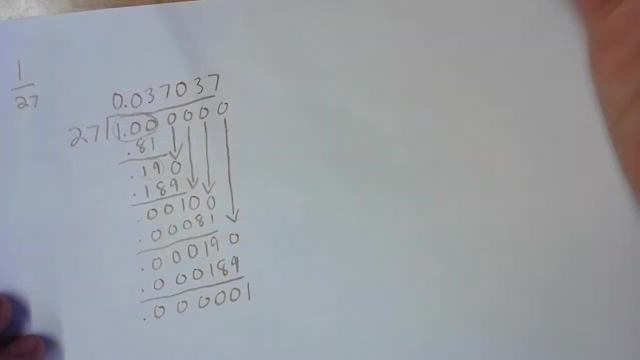 We remember from up here that it goes in 7 times, So 0.000189.. And then, once we do this process again, we will see that we are left at another 1.. A 0.0000001, but we're back at a 1, so we'll have to repeat the process all over again. 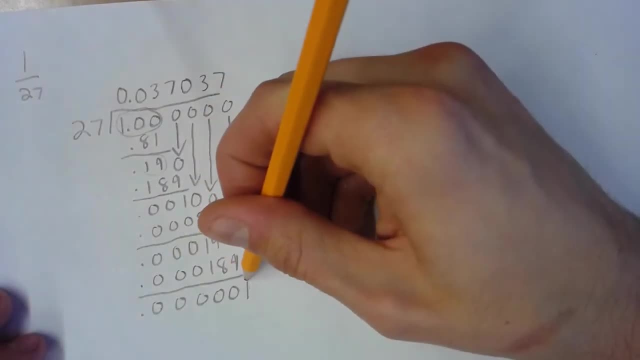 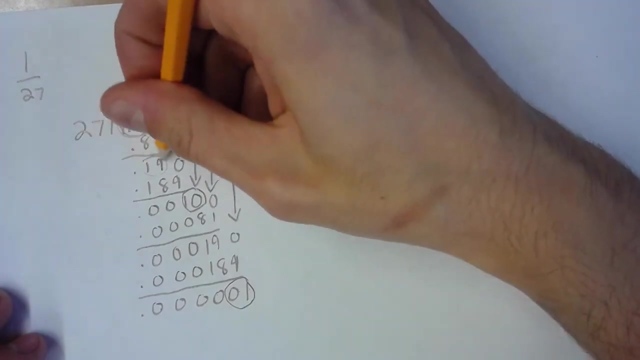 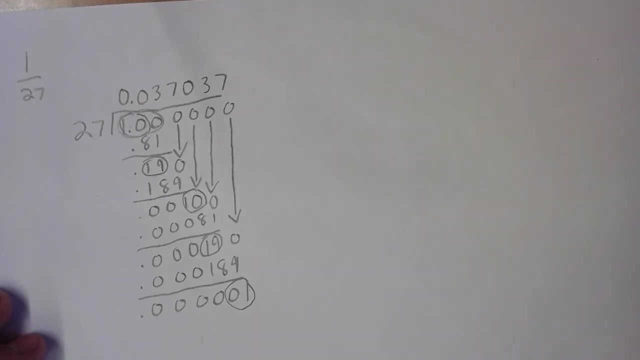 Now you'll notice something interesting about this problem. We tend to always go back to a 1 here. We also tend to see 19 a couple of different times, So this process is repeating. Where is the process repeating? Well, if we look at our answer up here here, we have a 0.03.. 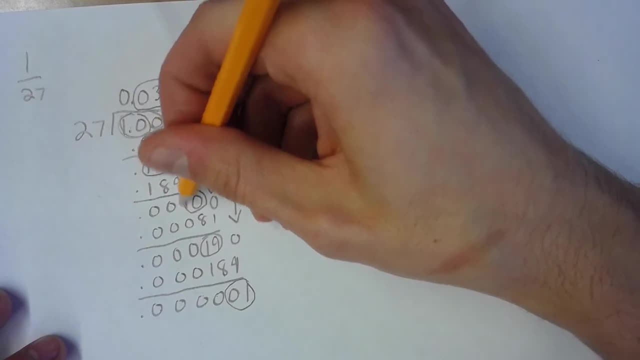 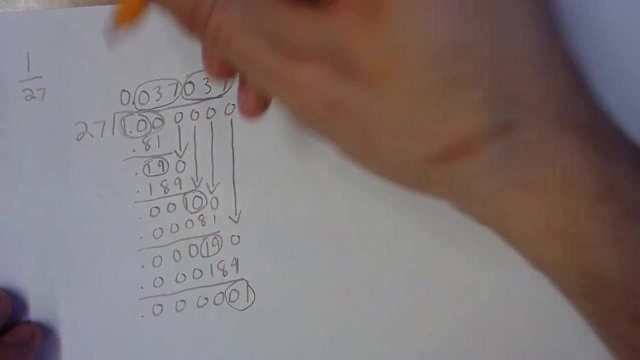 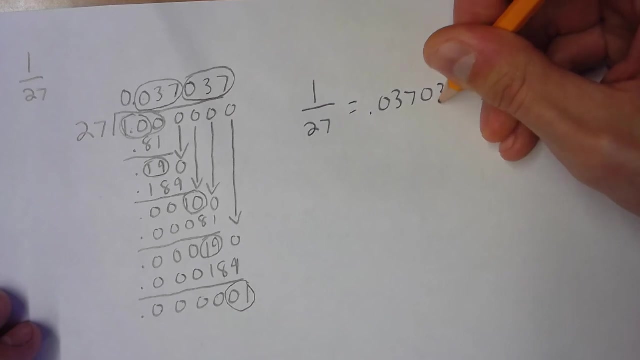 And then when we get back to our 1, right over here, we do another 0.037.. So here the repeating pattern is 0,, 3, and 7. And this is going to continue forever. So we know that 1 over 27, that is going to equal 0.037,, 0,, 3,, 7,, 0,, 3,, 7, going on forever.